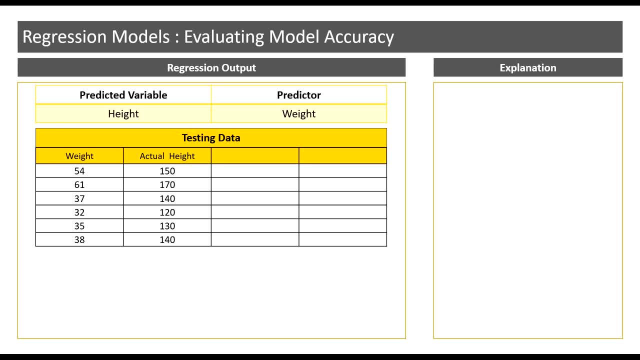 quick recap on training and testing data. Recall that the model will only be built on the training data set. Here the model will analyze the patterns in the training data set by understanding the relationship between the predictor and the predictor. The model will analyze the patterns in the training data set by understanding the relationship between the predictor. 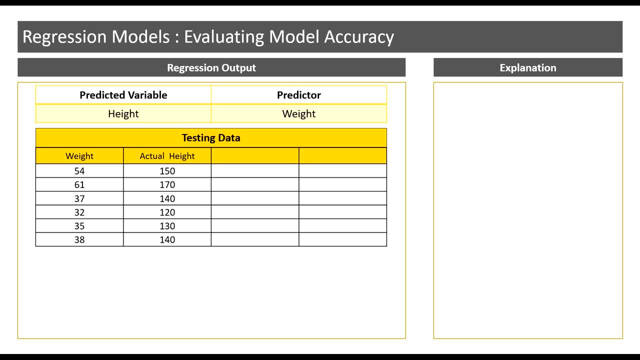 and the predictor, which in this case is weight and height respectively. The model will then go on to build a logic to predict height using weight as an input variable. As I mentioned in the previous videos, the model's accuracy will then be assessed on this testing data set. Here in the testing data set, we have values that are completely unexposed to the whole model building process. 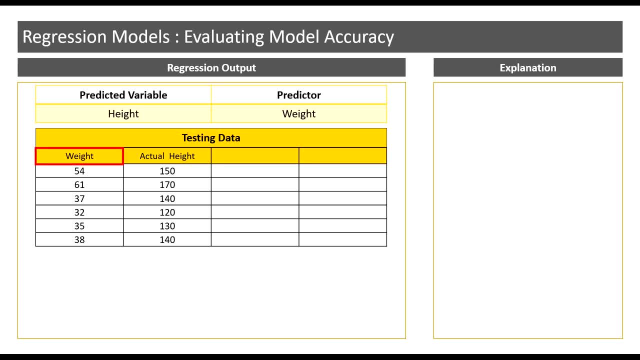 I will now pass the values of weight in the testing data set through the model which was built on the training data set to predict values for height. Then we will get the predicted values of height. Now we can compare the predicted values of height with the actual values of height in the testing data to see how far off our predictions were. 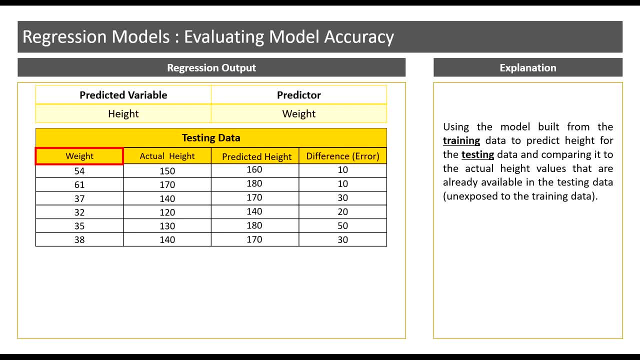 to begin with. We can go on to calculate the difference between the actual and the predicted values to understand the error in prediction. There are many measures to check for prediction accuracy, but it is important to note that all these measures stem from this error term right. 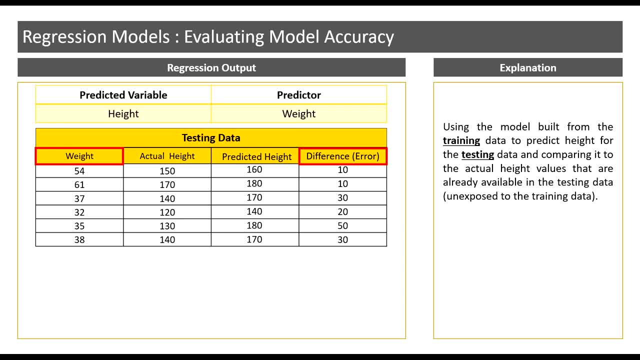 here. that is the difference between the actual and the predicted value. Now we will go through each of the error measures. The first error measure is mad ie Mean Absolute Deviation. It is calculated as follows: The formula is the sum of the absolute values of all the error terms divided. 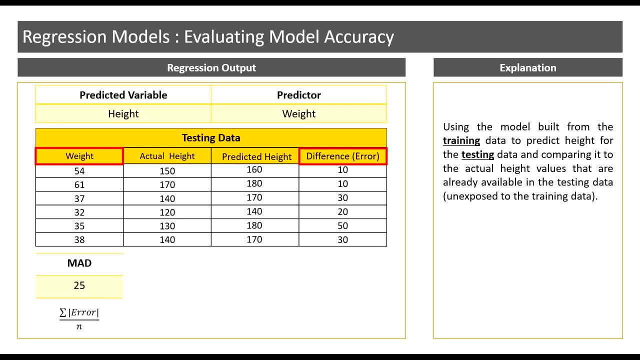 by the number of observations in the testing data set. The second measure is RMSE, ie Root Mean Square Error is calculated as follows. I will explain this calculation in two steps. Step 1, we first take the sum of the squared error terms and divide it by the number of observations in the testing. 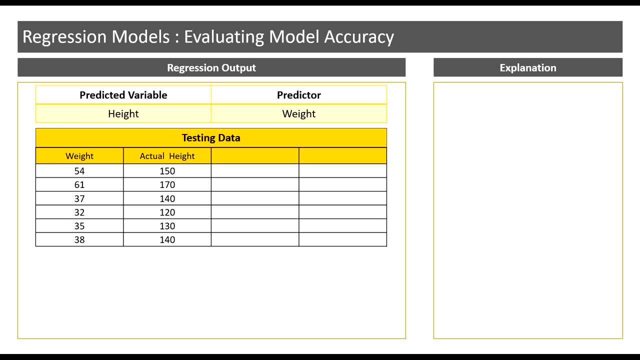 data set. Here in the testing data set we have values that are completely unexposed to the whole model building process. I will now pass the values of weight in the testing data set through the model, which was built on the training data set to predict values for height. Then we will get the predicted values of height. 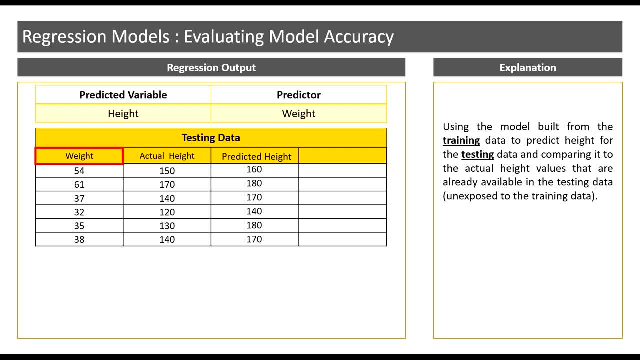 Now we can compare the predicted values of height with the actual values of height in the testing data to see how far off our predictions were. We can go on to calculate the difference between the actual and the predicted values to understand the error in prediction. There are many measures to check for prediction accuracy, but it is. 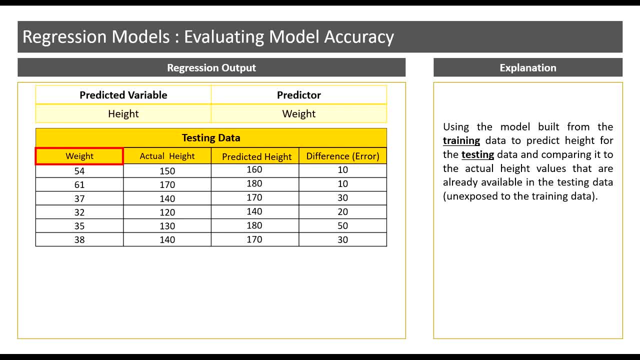 important to note that all these measures stem from this error term right here. That is the difference between the actual and the predicted value. Now we will go through each of the error measures. The first error measure is m a, D, that is mean absolute deviation. it is calculated as follows, The formula: 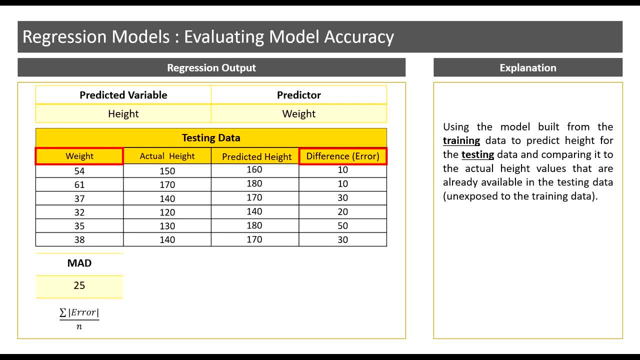 is the sum of the absolute values of all the error terms divided by the number of observations in the testing data set. The second measure is rms e, that is, root mean square error is calculated as follows. I will explain this calculation in two steps. Step 1, we first take 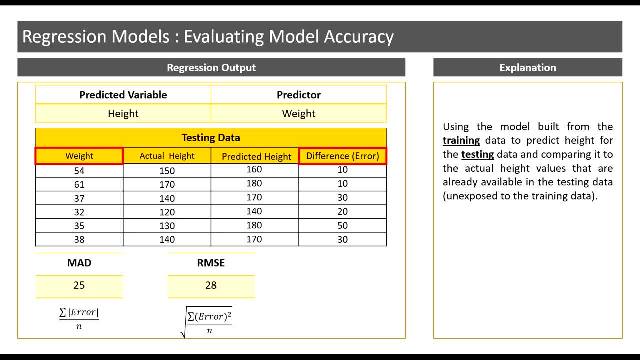 the sum of the squared error terms and divide it by the number of observations in the testing data set, Step 2, we then take the square root of the value obtained from step 1.. Now the third and the last measure, which is MAPE, that is, mean absolute percentage error. Note that since this 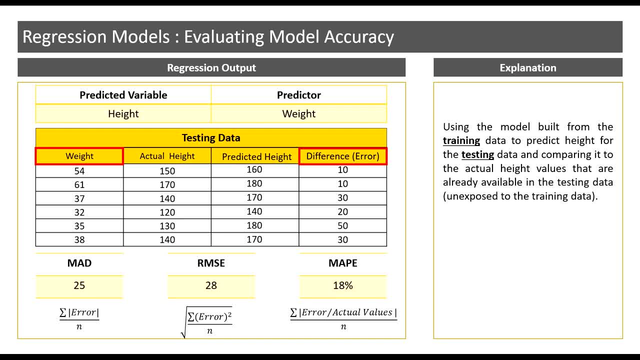 error is in percentage, it becomes a relative measure. The calculation for this measure is as follows: It is the sum of the absolute values, of the ratio of the error terms and the actual values divided by the number of observations in the testing data set. Now please don't get worried. 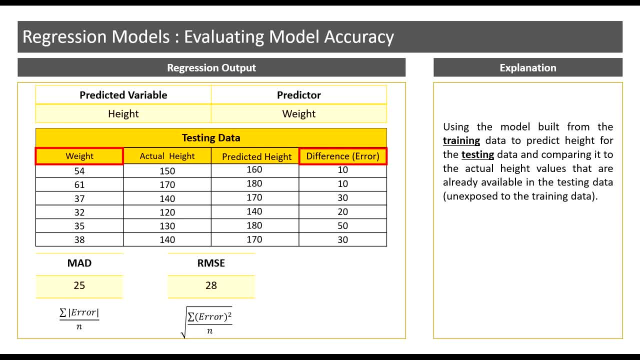 data set, Step 2, we then take the square root of the value obtained from step 1.. Now the third and the last measure, which is MAPE. that is mean absolute percentage error. Note that since this error is in percentage, it becomes a relative measure. The calculation for this measure is as: 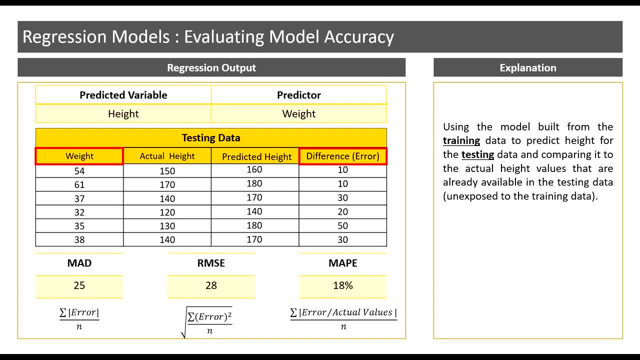 follows. It is the sum of the absolute values, of the ratio, of the error terms and the actual values divided by the number of observations in the testing data set. Now please don't get worried, or don't even bother to remember these formulas, because R has many packages and functions that 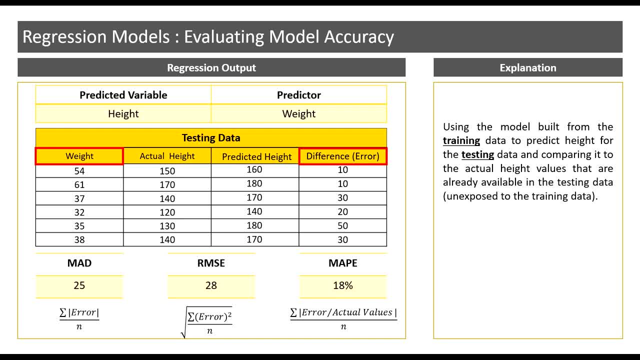 will help calculate all these measures. More than remembering the formula, I want all of you to understand how these measures are interpreted as such. So how do we interpret these measures? So I predicted height here and note that height is in centimeters. Therefore, values such as MAD. 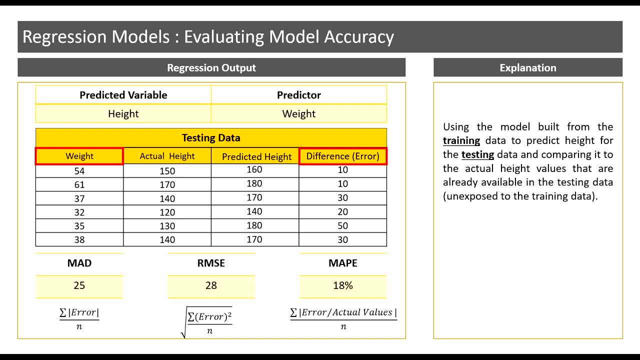 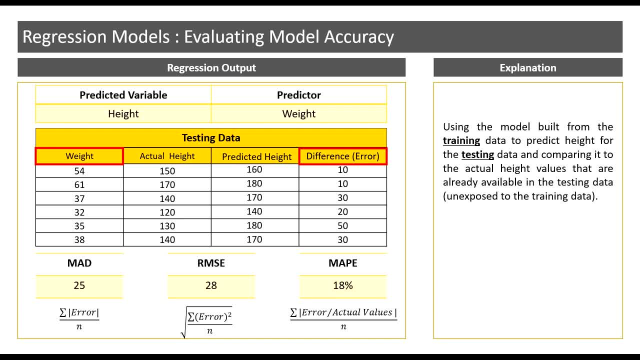 time when I use this model to predict height, I may be off by roughly 25 centimeters. That is, the predicted value could be 25 centimeters above or 25 centimeters below the actual value. Now let us move on to RMSE. Here we see that the RMSE is 28.. Here it suggests that next time 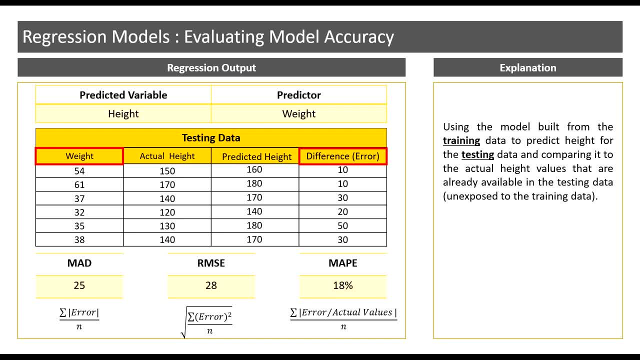 I use this model to predict height. I may be off by approximately 28 centimeters. So the RMSE is similar to MAD, but it penalizes the model further. In other words, it is just a stricter measure. Now let us move on to our last measure, that is, MAPE. As I mentioned before, the MAPE is a relative 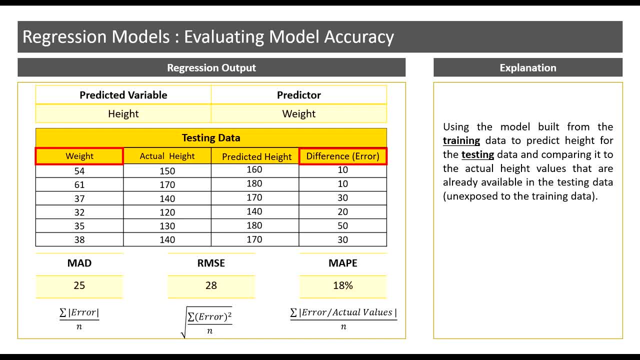 measure, It expresses the error as a percentage. Therefore, when we say that the MAPE is 18 percent here, it suggests that this is a positive, that next time I predict height I would be nearly off by about 18 percent. that is, I would be either. 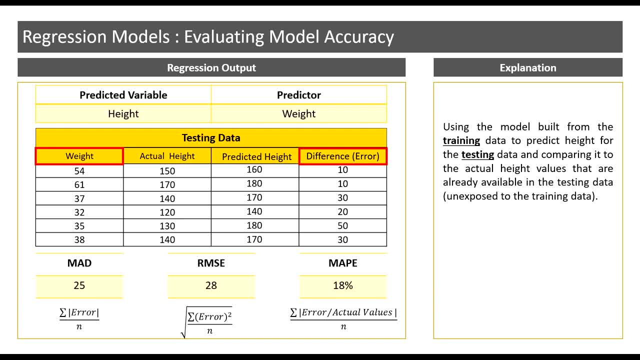 or don't even bother to remember these formulas, because R has many packages and functions that will help calculate all these measures. More than remembering the formula, I want all of you to understand how these measures are interpreted as such. So how do we interpret these measures? 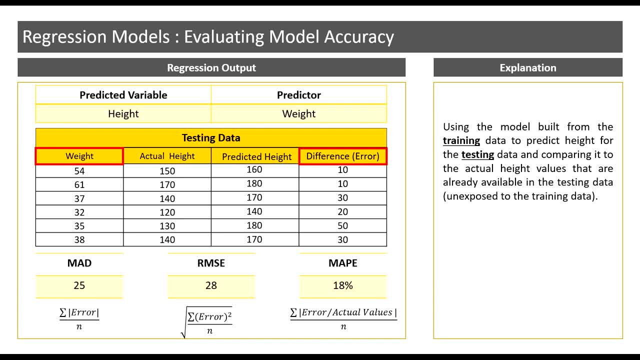 So I predicted height here and note that height is in centimeters. Therefore, values such as MAD and RMSE will also be in centimeters, as these error measures are on the same scale as the value of MAPE. Now let's see how we can interpret this in centimeters. So 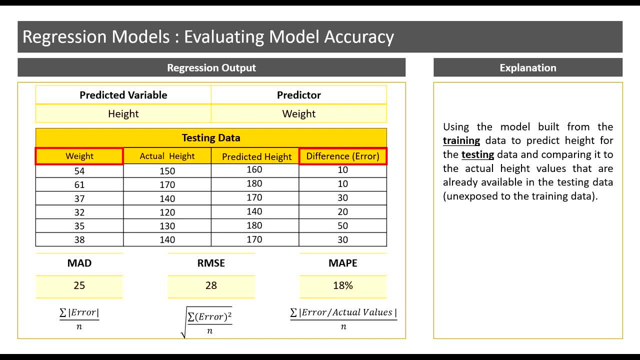 scale as the predicted variable. So when we say that the MAD is 25 here, it suggests that next time, when I use this model to predict height, I may be off by roughly 25 centimeters, That is, the predicted value could be 25 centimeters above or 25 centimeters below the actual value. Now let us 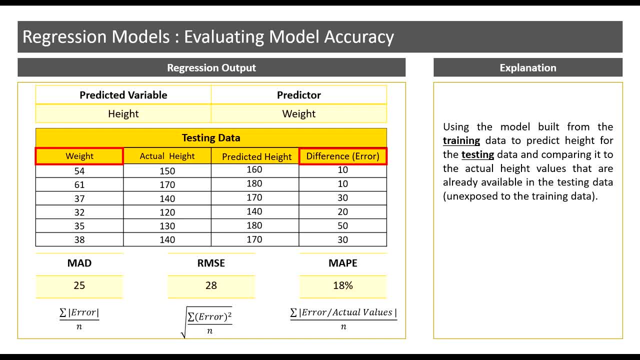 move on to RMSE. Here we see that the RMSE is 28.. Here it suggests that next time I use this model to predict height, I may be off by approximately 28 centimeters. So the RMSE is similar to MAD, but it penalizes the model further. In other words, it is just a stricter measure. Now let us move on. 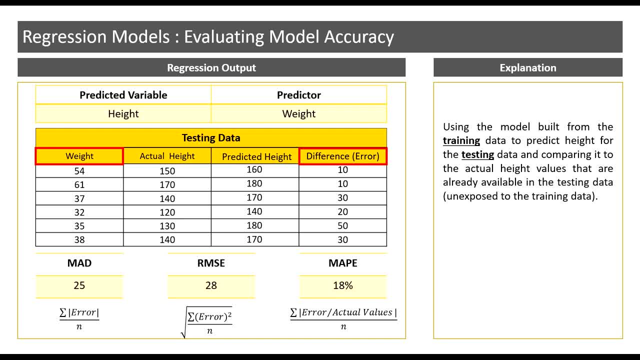 to our last measure, that is, MAPE. As I mentioned before, the MAPE is a relative measure. It expresses the error as a percentage. Therefore, when we say that the MAPE is 18 percent here, it suggests that next time I predict height, I would be nearly off by about 18 percent. That is, I would be either 18. 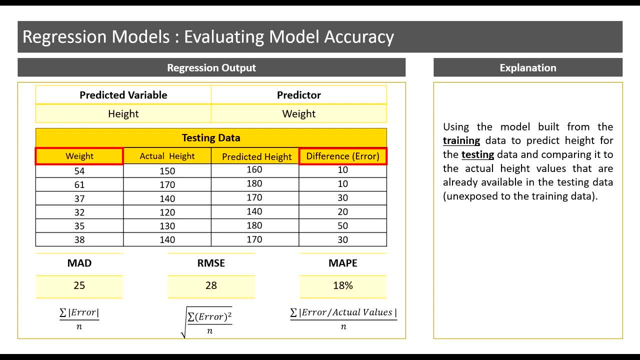 percent above or below the actual height value. Now, when it comes to all these measures, which is preferable? Well, I personally prefer MAPE, and I'll tell you why. Once I was working on a case where I had to predict sales for an for an airline, which was a little bit more expensive, So I had to. 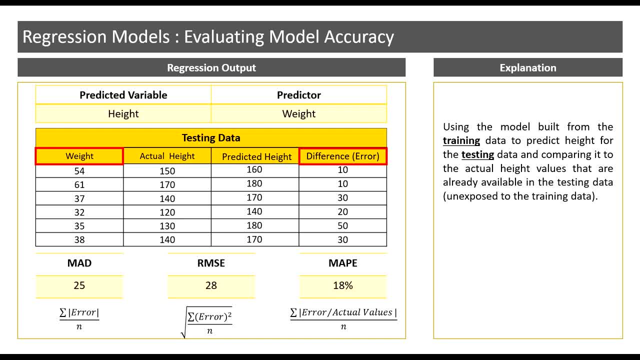 predict sales for an airline which was based out of Germany, I got an RMSE value of 150,000.. Now this value seems very high, right? So this is because the predicted sales value was in millions of euros. So if I had predicted the sales to be 1 million euros- and I'm off by about 150,000 euros now- this